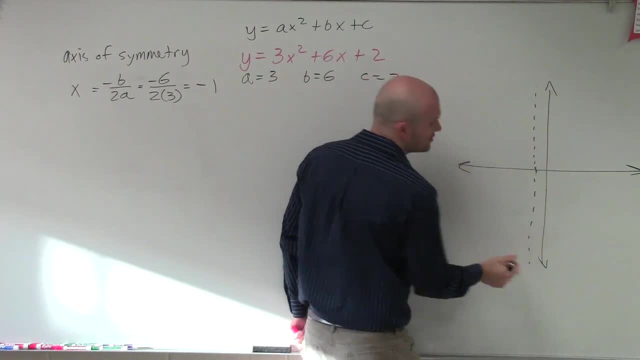 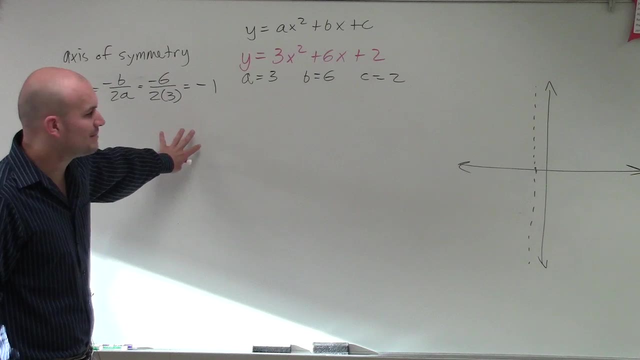 a vertical line, But I'm going to make it dotted because it's not actually going to be a part of my graph. It's going to be the line that my graph is going to be symmetrical about. So, now that I've found my axis symmetry- remember when we find the axis symmetry, it's very, very important about. 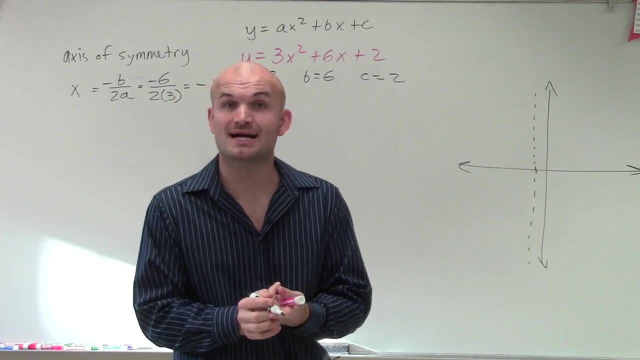 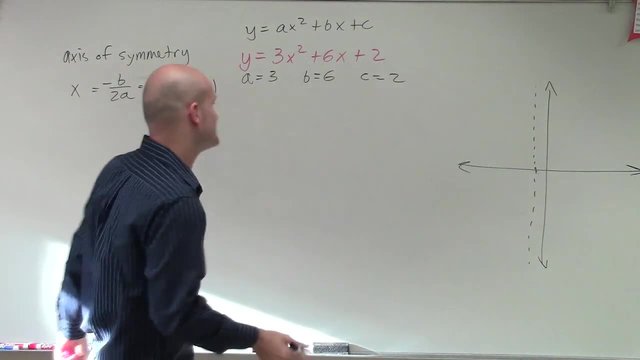 finding the axis symmetry, because one our vertex goes through our axis symmetry, And then also all the points to the left of the axis symmetry. we can now reflect over the axis symmetry to create the points on the right. So what I'm going to do is I'm just going to pick. well, first, 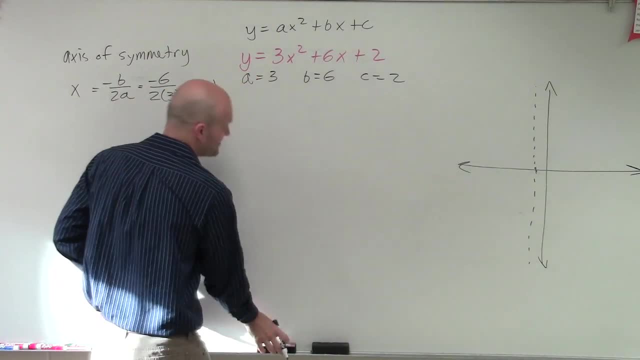 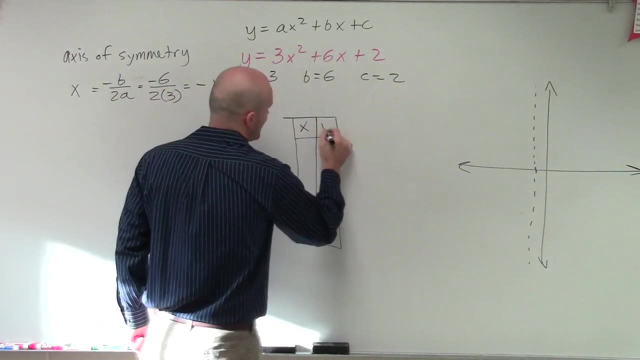 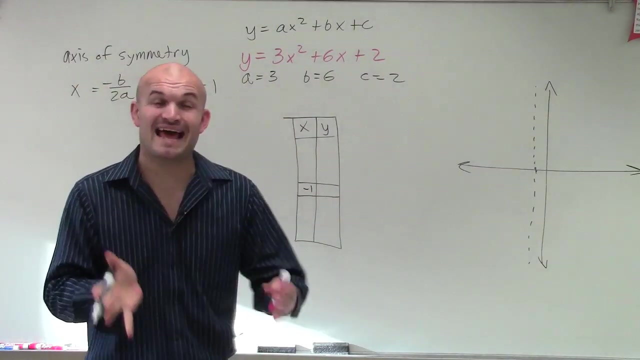 what am I doing? I want to create a table of values, not another graph. So what I'm going to do is I'm going to make a table of values And I'm going to pick three points. And the first point I'm going to pick for my y x-coordinate is going to be the vertex right, Because we know that the 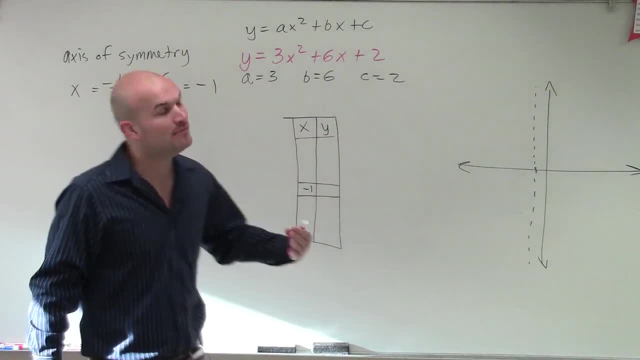 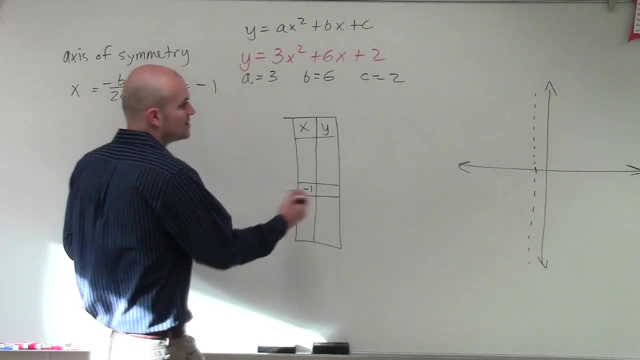 axis of symmetry. So I'm going to evaluate for negative 1, and then what I'm going to do is I want to pick two points, either to the left or to the right, to find those values, and then I'm going to reflect them over the axis of symmetry. So I'm going to pick two points to the right, So I'll do. 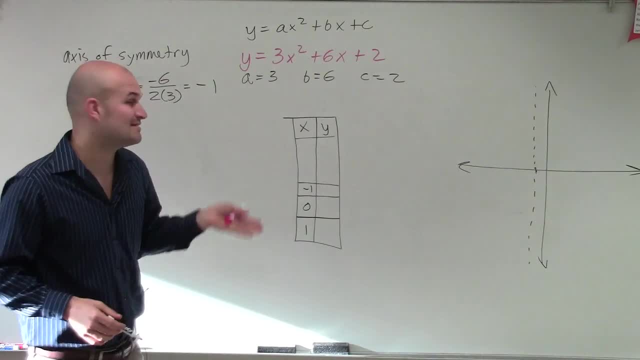 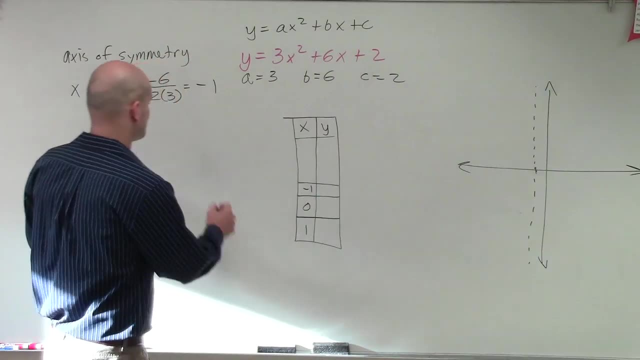 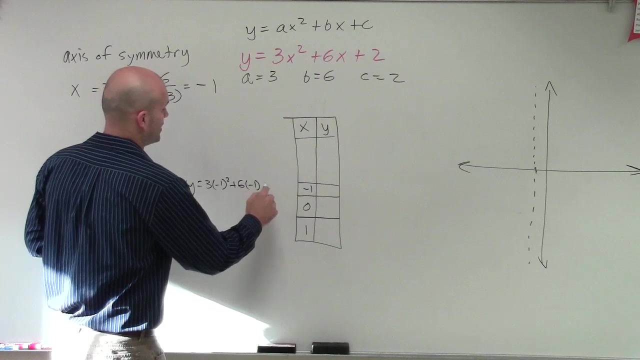 0 and 1.. Now what I'm going to do is evaluate them. So these are the x-coordinates of my point on the quadratic, and now I need to be able to figure out what the y-coordinate is going to be. So I'll just do the first one. y equals 3 times negative 1 squared plus 6 times negative 1. 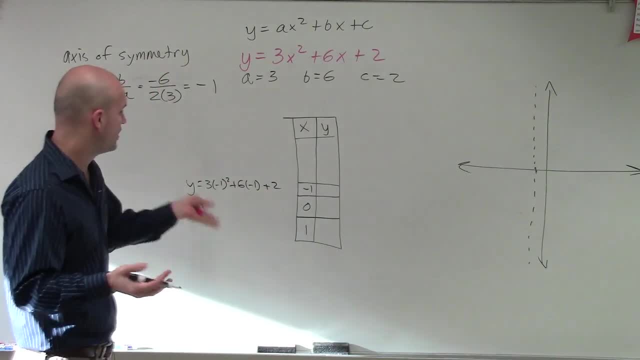 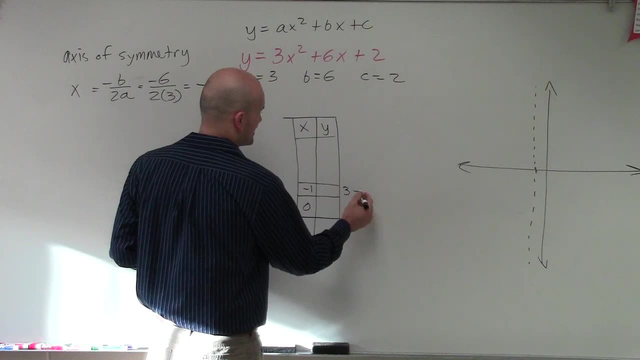 plus 2.. Well, negative 1 squared is 1,. 1 times 3 is 3, plus 6 times negative 1 is a negative 1, so we'll just do- or sorry, negative 6, so we'll do 3 minus 6, and then plus 2, and that gives us: 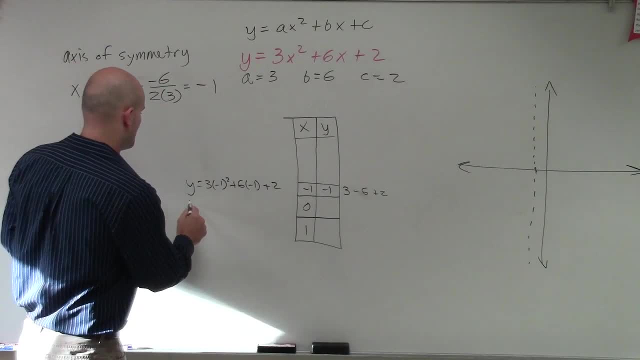 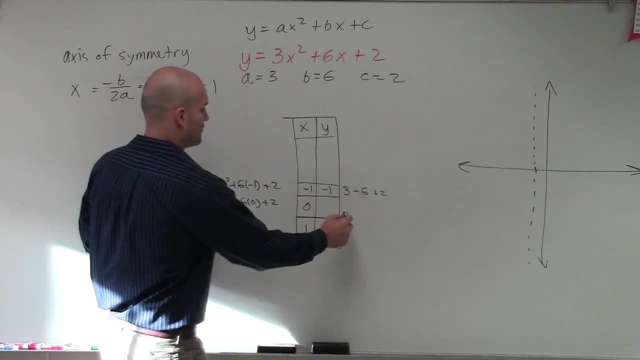 a point of negative 1.. Now let's do 0, so y equals 3 times 0 squared, plus 6 times negative 1, 6 times 0 plus 2, so therefore I have 0 plus 0 plus 2, which is now going to be 2, and then I 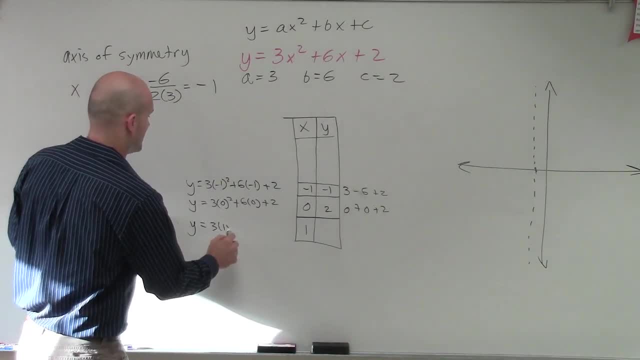 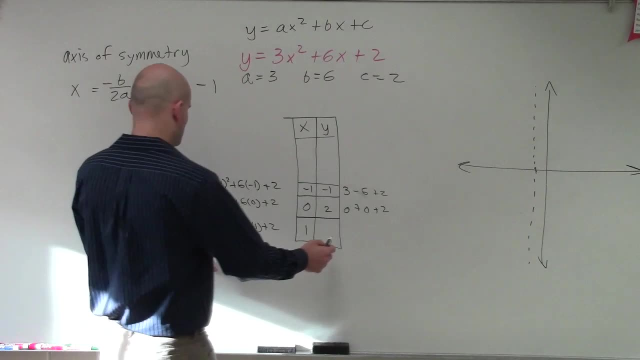 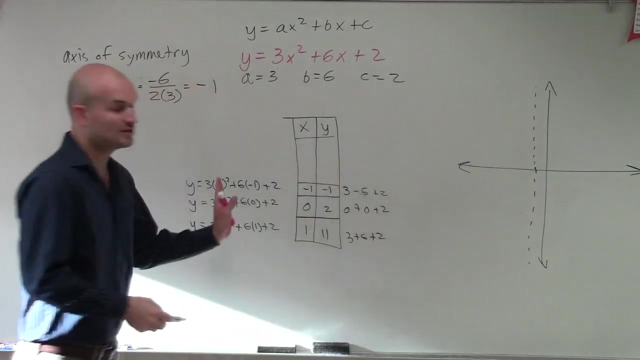 have 1, so I have: y equals 3 times 1 squared plus 6 times 1 plus 2.. 1 squared is 1 times 3, is 3 plus 6 plus 2, so that's going to be 9, that gives me 11.. So these are going to be by two points to. 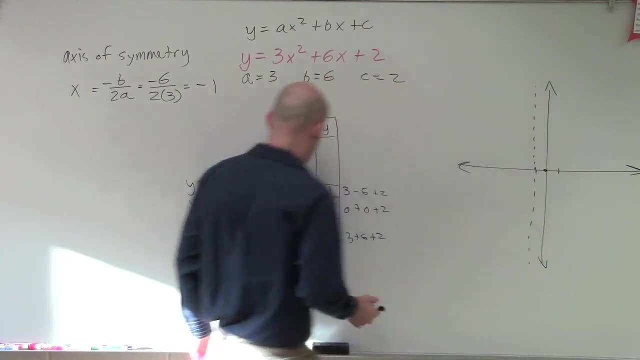 the right. so I have negative 1 squared plus 6 times 0 plus 2, so I have 1 squared plus 6 times 0 squared plus 6, so I have 0 and 1, and if I was going to do two points to the left, what I'm? 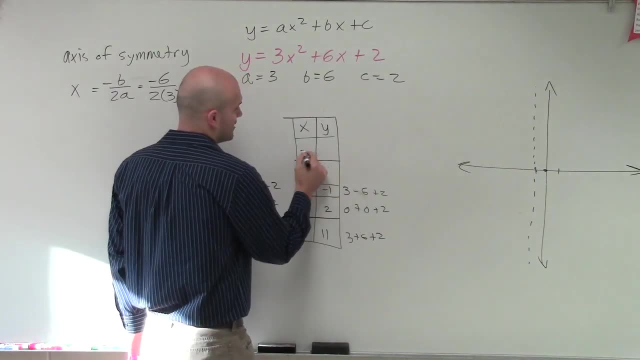 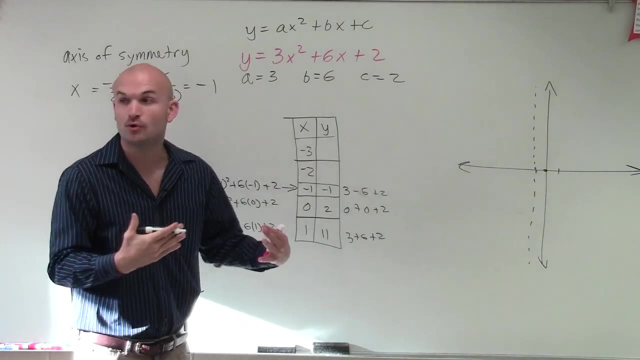 going to reflect about that would be negative 2 and negative 3.. Now, remember, here's my axis of symmetry. right, My graph reflects over my axis of symmetry, and let me just kind of show you what these points are, so then you can see it and then I'll fill in the table. So my vertex is at: 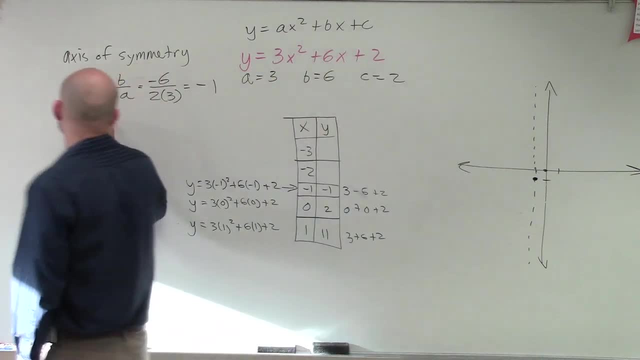 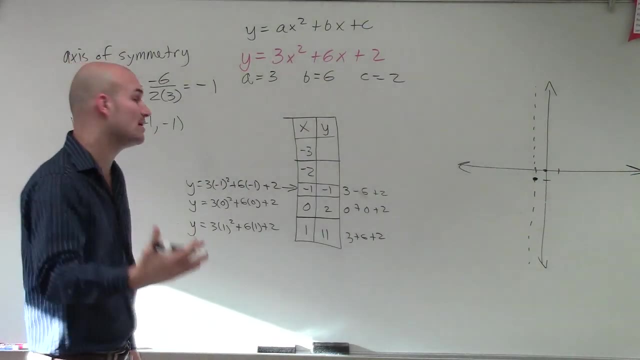 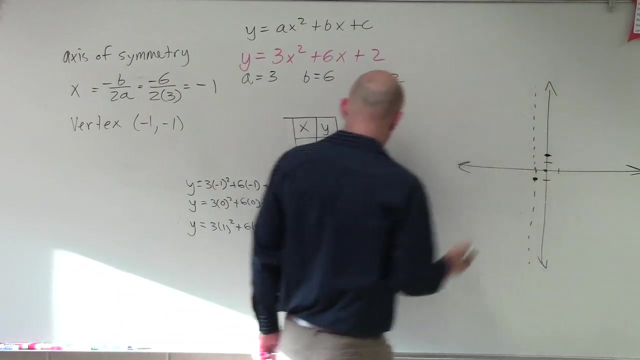 negative 1, negative 1.. So now I can just write: my vertex is going to be at negative 1, negative 1.. That's going to be the minimum point on my axis, My graph. Then we go and look at 0, 2, so 0, up 2, and then 1, 11.. So over 1, up 1, 2, 3,, 4,, 5, 6,, 7,, 8,, 9,, 10, 11.. 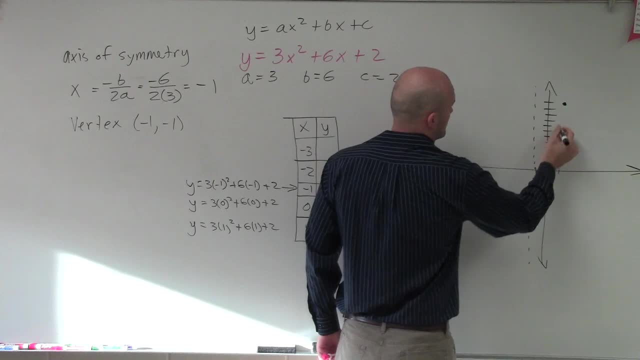 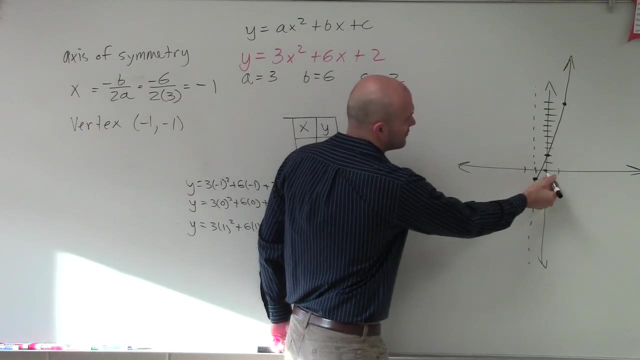 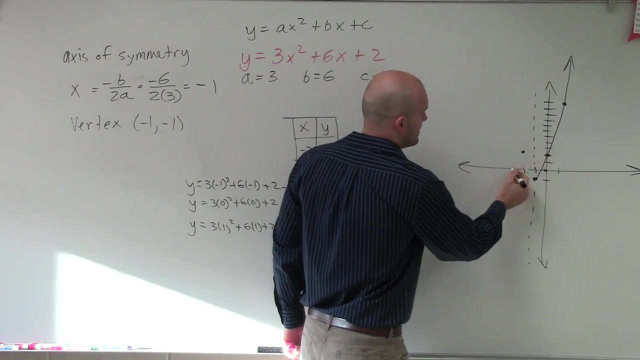 So you can see, my graph is starting to look like this. but remember, this is my vertex. so what's going to happen is now when I reflect it over my axis of symmetry- I'm sorry that goes up there- and then when I go over 2, it comes up to here. so my graph's going to follow a path like this. 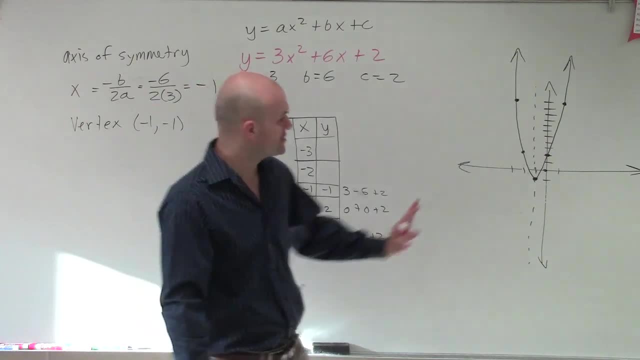 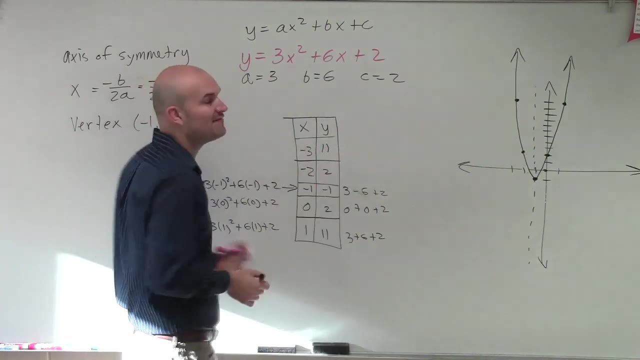 So why it's so important to find the axis of symmetry? because, rather than plugging in all these points, I know that negative 2 is going to give me 2, and I know that negative 3 is going to give me 11 by 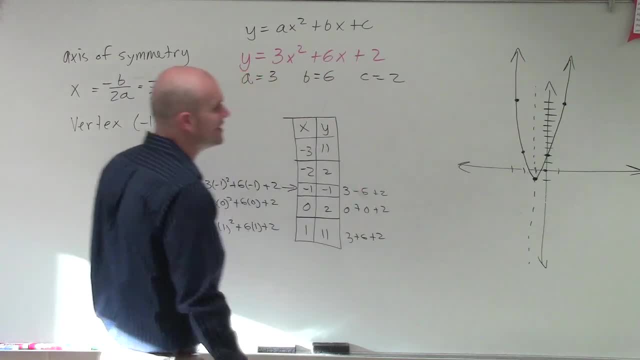 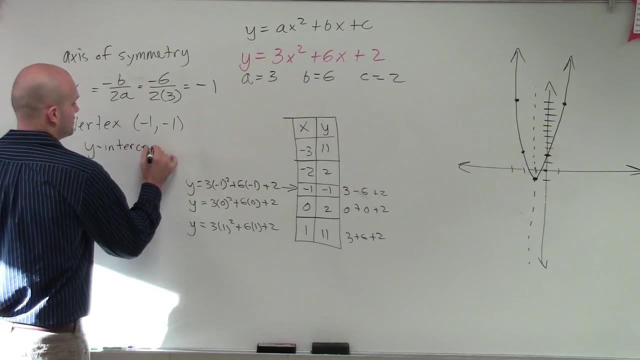 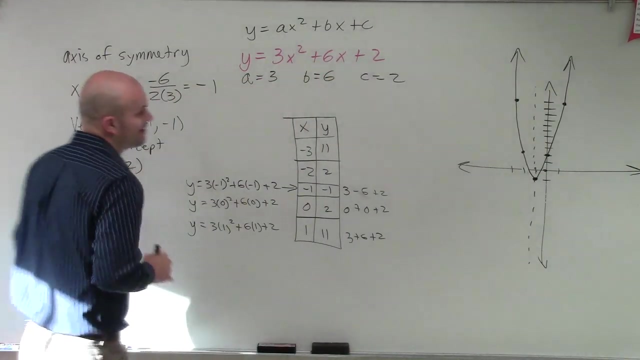 applying my axis of symmetry. Now the next thing is we need to kind of determine our x and y-intercepts. So our y-intercept is where the graph crosses the y-axis. Well, you can see here, the graph crosses the y-axis at 0,, 2, and the x-intercept is where the graph 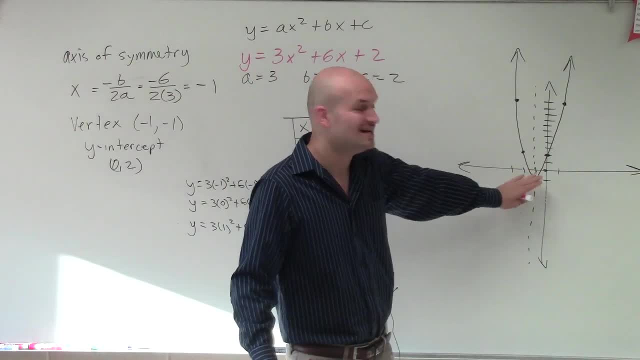 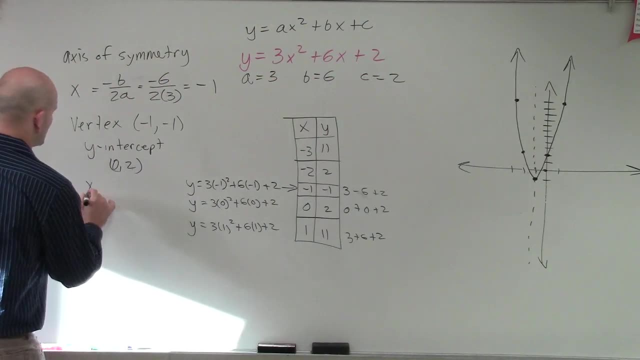 crosses the x-axis. Now it doesn't look like it crosses it at its integer. so right now I'm just going to estimate and we'll learn later on how to find this exact value. So the x-intercepts I'm just going to say is going to be between negative 2 is less. 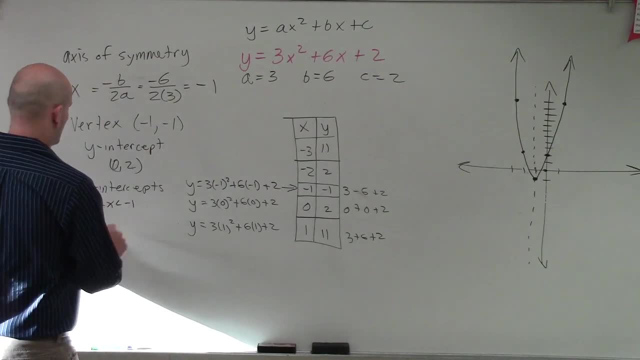 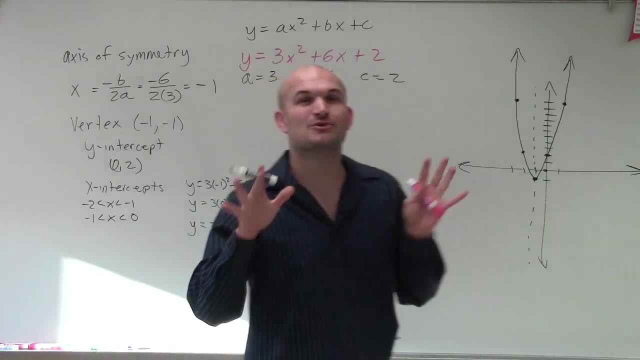 than x, which is less than negative 1, and then we have negative 1 is less than x, which is less than 0.. So our values are going to be somewhere in between there and, like I said, I'm just going to estimate for right now and then we'll show you how to find those.